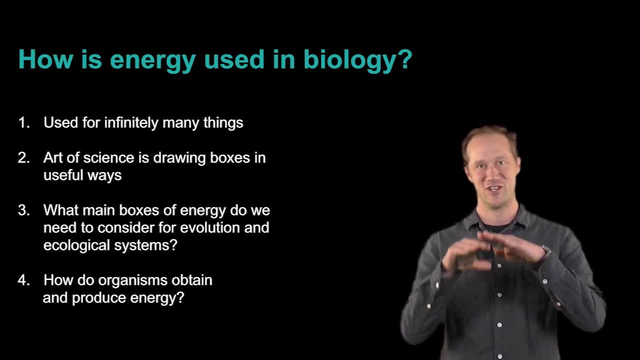 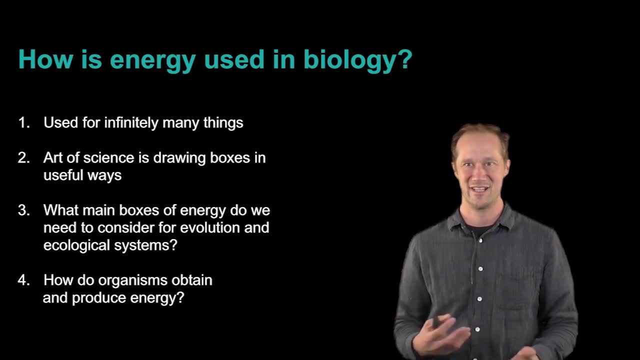 to me, and one of the arts of science to me, is deciding how to draw the boxes that we're going to use, And to do that you often have to frame a question or think about some objective you're trying to meet. And the two I'm going to talk about in this talk- one is with relation- 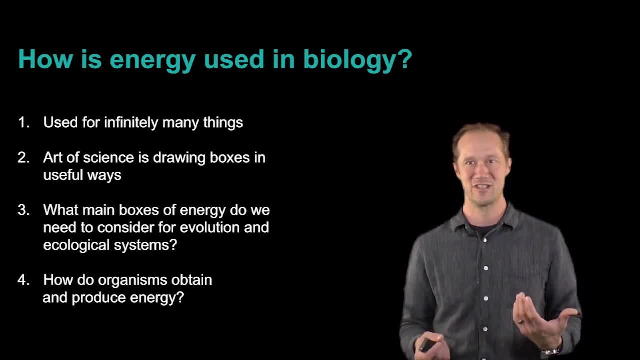 to evolution- How do we think about energy in terms of evolution and what's the need for evolution? And the other is more in relation to physiology and ecology, which really has to do with how do we get energy and how do we make energy. 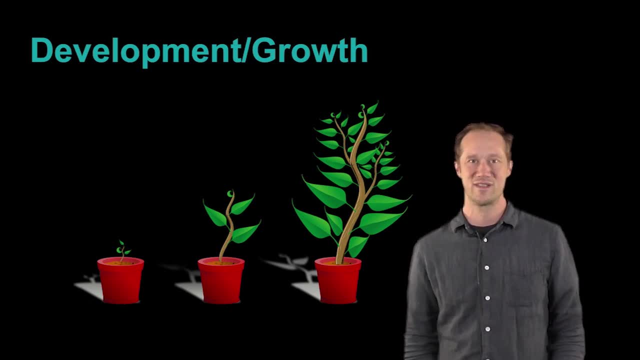 So from an evolutionary perspective, the main thing we are concerned about is fitness, which is how many offspring or individuals we give to the next generation. And to do that we first have to grow and maintain ourselves to reproduce. So one of the main boxes for evolution actually is development and growth. So in this slide I show a plant. 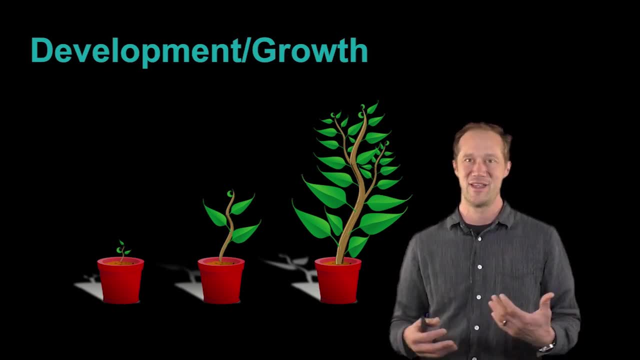 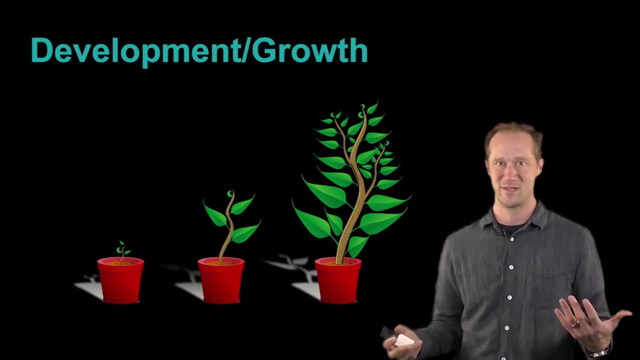 growing from early stages to later, And in doing that it has to create many more cells. It has to create new types of cells and new types of structures. So this takes a lot of energy and is a very energy-intensive process, And that's also true for animals and their growth. Here there's a picture of these two. 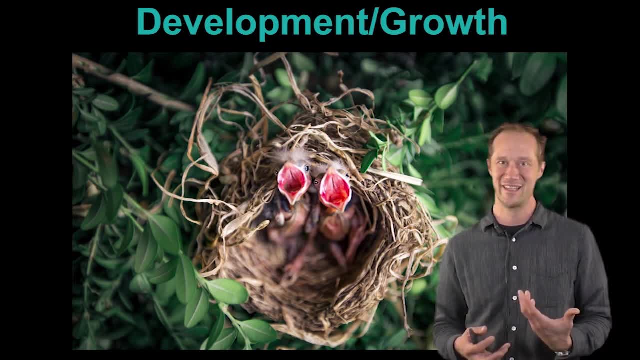 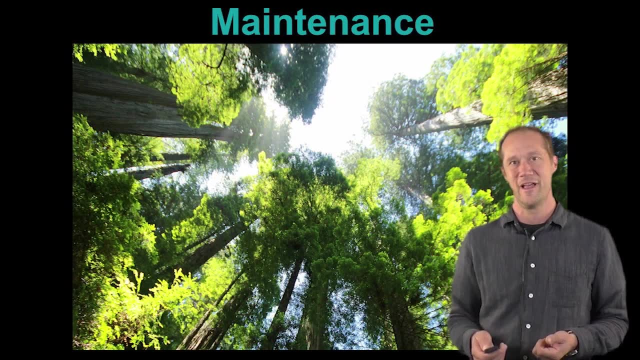 birds crying out to their parents. They're crying out to their parents for food, to bring them food, because they need lots more food to grow and have energy to be big enough to reproduce. The next box I'll talk to you about for energy is maintenance And that's sort of a less. 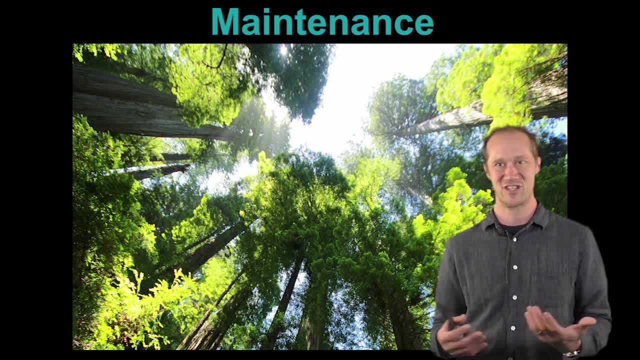 obvious, visible one, because you're not seeing cells change or structures change or reproducing. You sort of see things staying the same way. they are visibly, but actually that takes a lot of energy just to replace cells that die or to feed cells energy just to keep living. 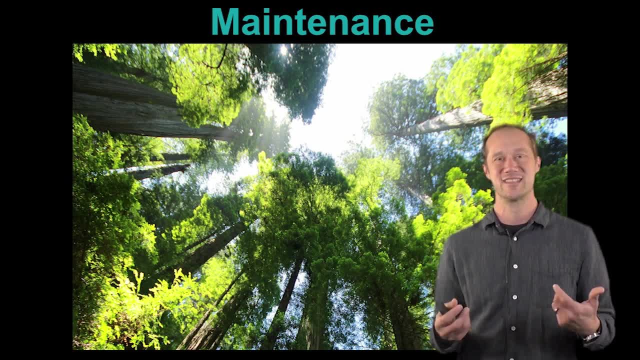 Those extreme examples. if you look at these redwood trees, it takes an enormous amount of energy just to keep water or sap pumping up to the leaves at the top. It's a huge distance they have to travel and you have to build structures to maintain them. to go up to these. 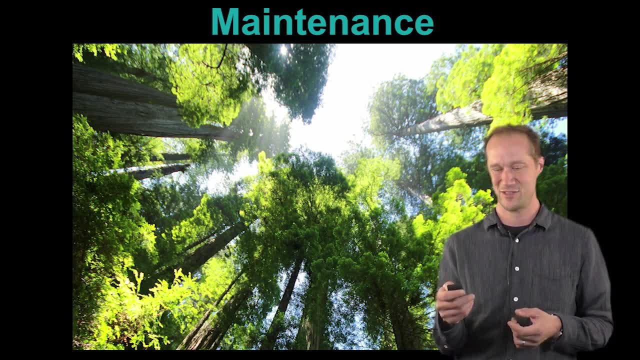 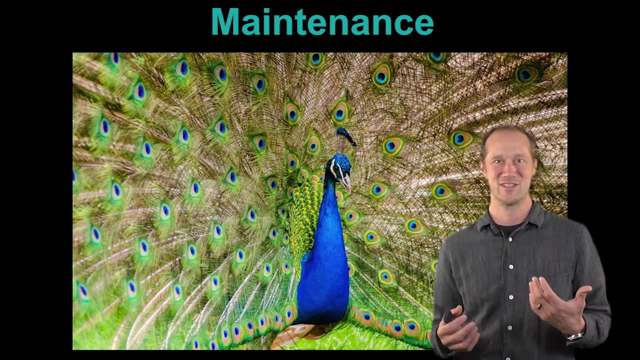 leaves. So you use a lot of energy just to keep pushing up to the tops of the trees, And similarly we use energy for all the structures in our body. but there are extreme examples here too. If you're thinking about a peacock, if it builds a whole array of feathers, it's going. 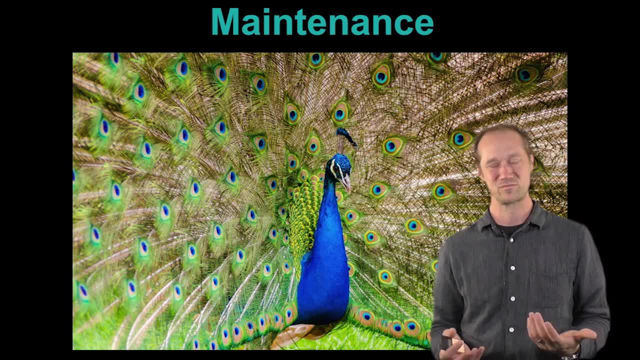 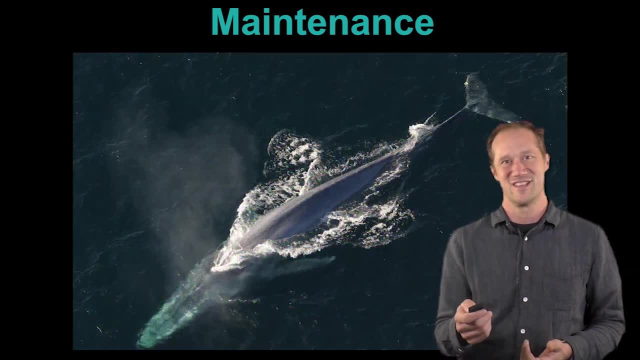 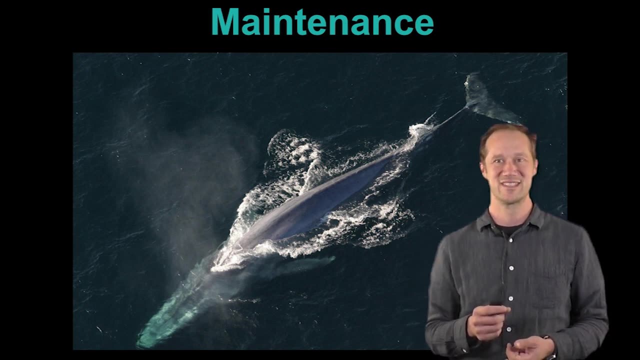 to need a lot of energy to build and to maintain and it's going to use that to attract a mate, which again it needs for reproduction, which is important for evolution. So, as a brief aside before I get to reproduction for maintenance, one of the things to me about, 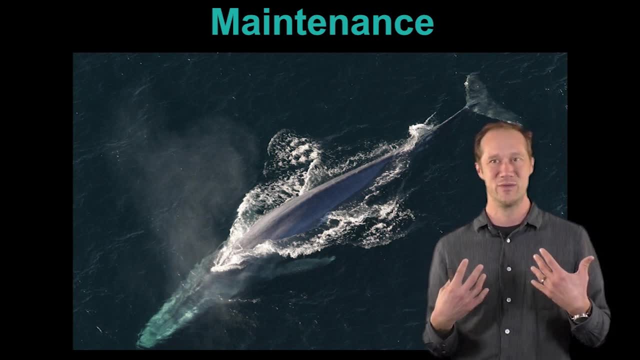 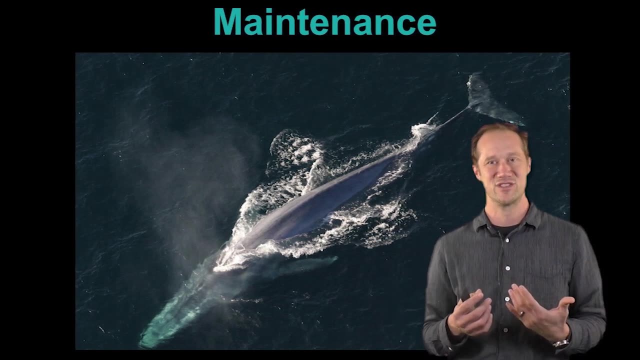 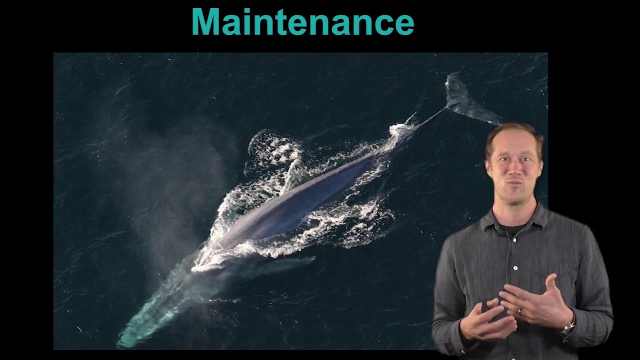 us as humans is that individually, biologically, we use about the same amount of power or energy per time that you would see in a light bulb. But once you add in things how much energy we use for a car Or computers or light bulbs or heating our houses, we actually, each individual in the 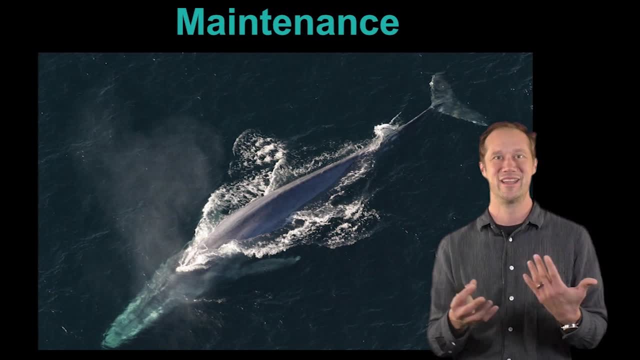 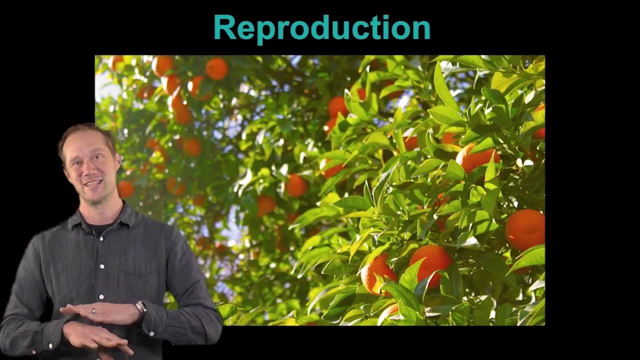 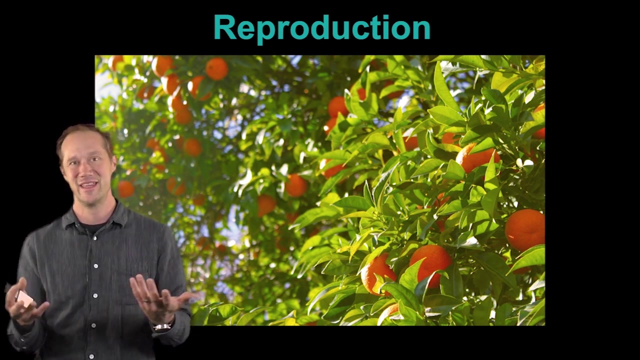 US uses about the same amount of energy as a blue whale, So we're really enormous energy users in terms of our biological footprint. The last evolutionary box I'll talk about for energy is reproduction, which is where evolution is ultimately aimed most of the time, And that can be things like oranges. 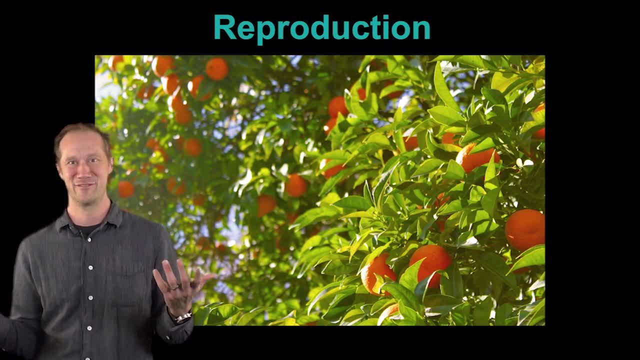 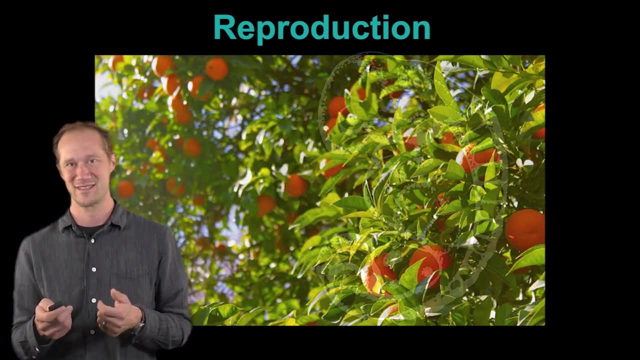 on a tree that tempt us to eat them because they're so pretty and flavorful and taste good. And then we walk around and distribute those seeds to help orange trees grow elsewhere and increase their numbers. Or also an embryo growing inside a mother. that takes a huge. 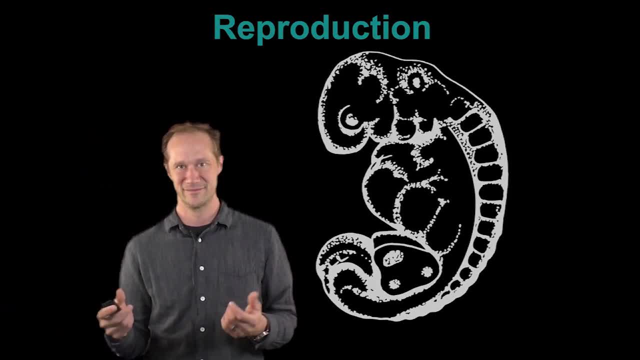 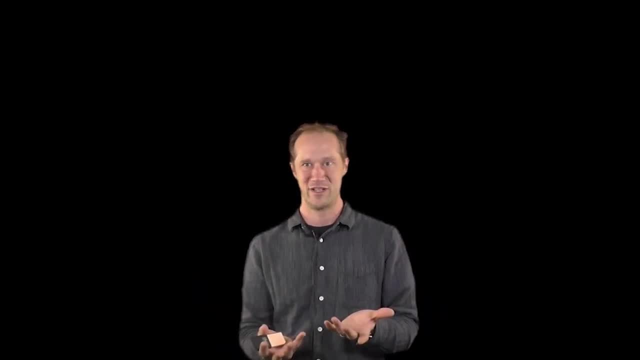 amount of energy and time to produce that's necessary for reproduction. So growth, maintenance and reproduction are the main boxes I think you can think about for evolution, where energy is needed. But now I'm going to shift gears and talk a little bit more about how it's needed for physiology and ecology, which has a lot to do with how 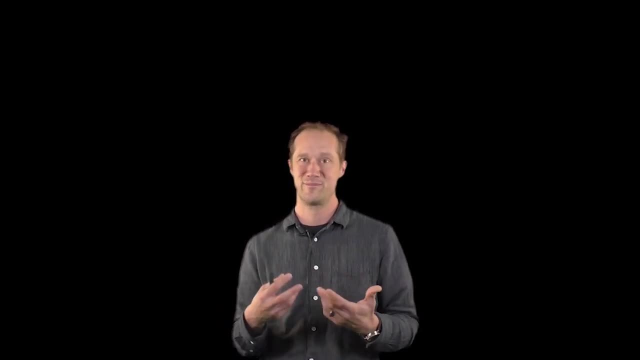 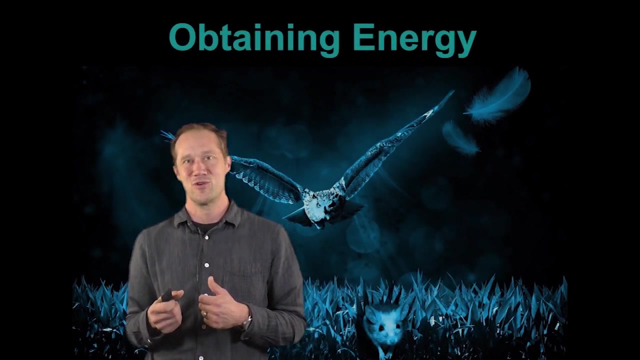 you get energy and how do you make it, Which evolution still plays a big role in, because you need those things to survive- but it's not as explicit as if you do it this way. So, in terms of obtaining energy, this is a dramatic picture of an owl chasing down a. 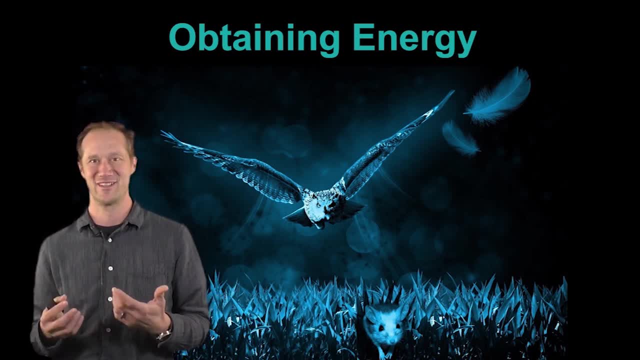 mouse to eat for food, And that's one type of example of getting resources or food is through what we call active capture, But other ways include things like grazing like a cow in a pasture or sit and wait, which would be like snakes or spiders waiting for prey. 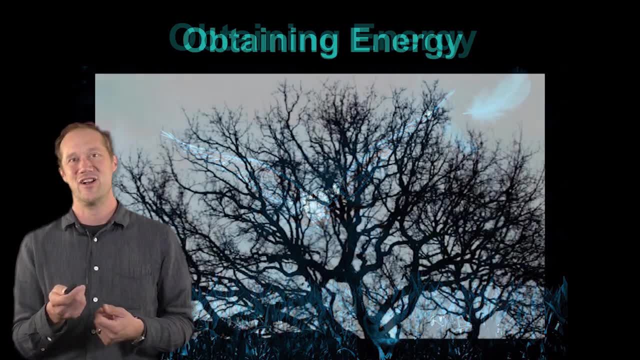 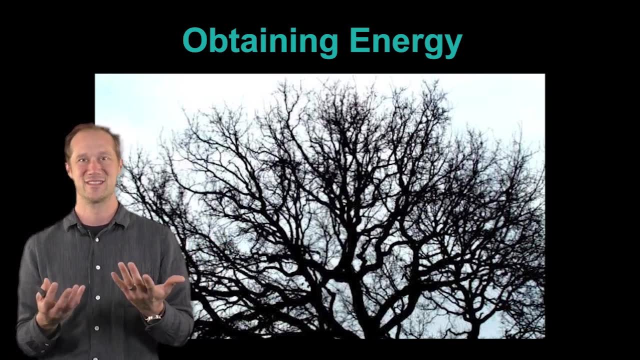 items to come to them. And also plants are a little bit like that in terms of getting energy. They're more like sit and wait, where they build structures and wait for things to come to them. So, as we see here, there's an extensive branching system for this tree, And when the leaves 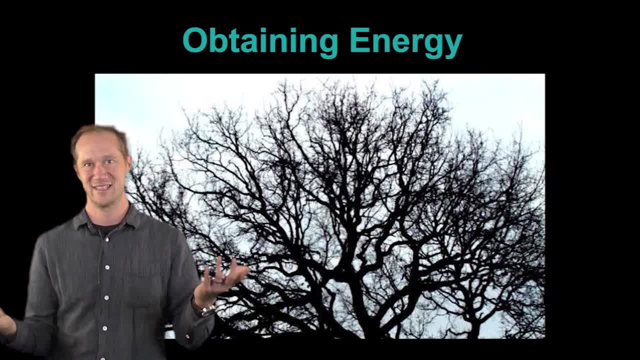 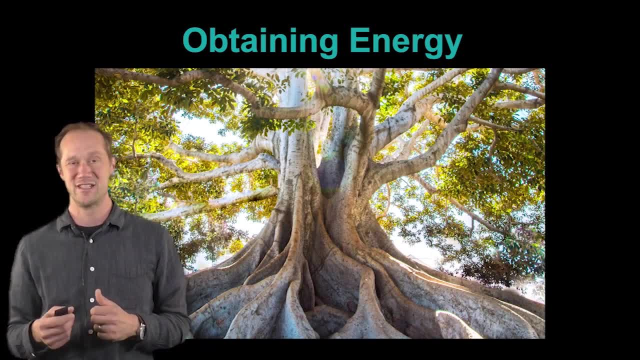 are all present on the limbs. it's using that to get light, to get light from the environment and get as much light in this little area as it can within that canopy And that sort of branching system is reflected below ground in terms of root systems. that 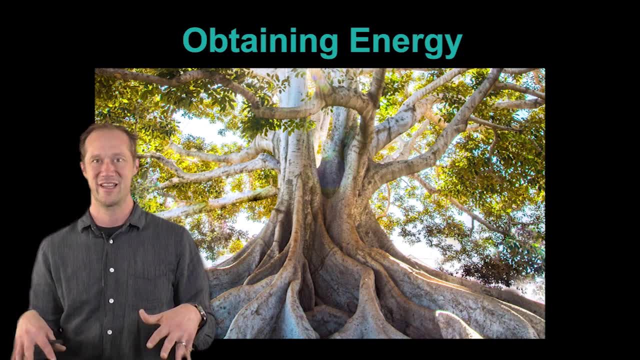 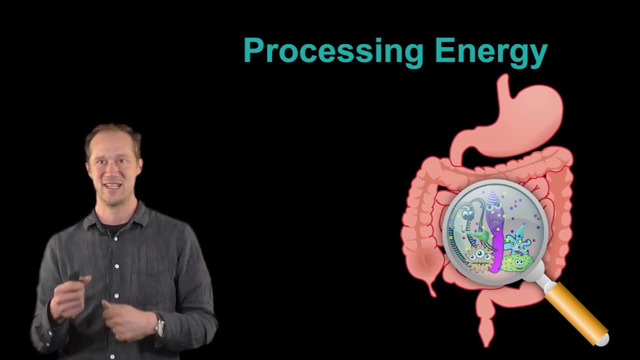 it uses to get water and nutrients from the ground as well, where it has to branch out and get as much resources as it can. Once resources are obtained, we have to process that to make energy, And the first step in that for animals is the digestive system, which involves going through our stomachs. 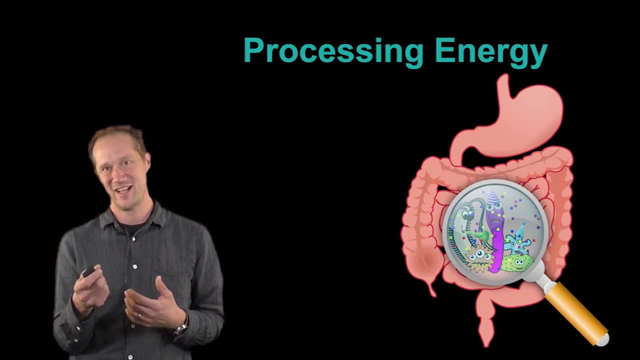 and things like that. But the part I want to highlight here is that in our guts there are these microbial systems, often now called the microbiome, gut microbiome- which we have to have to process energy. It's this own little world and ecosystem inside our bodies. 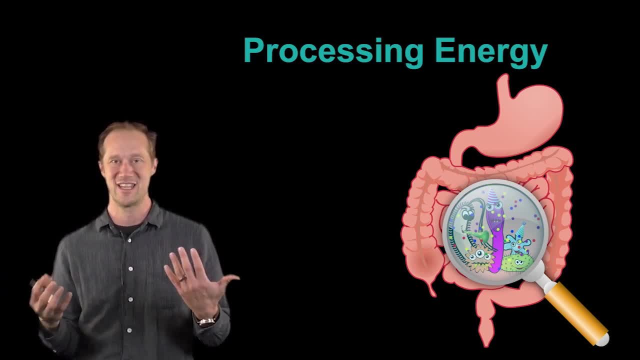 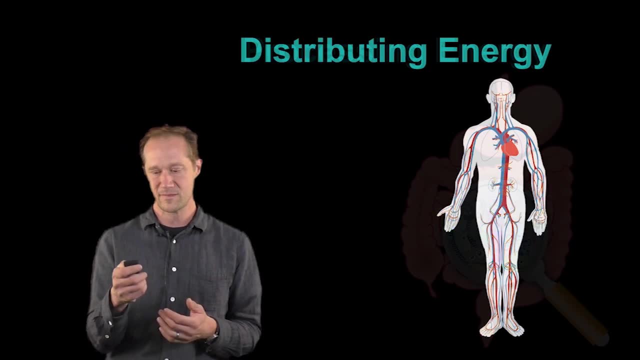 And basically based on how it processes energy and the energy needs. it really affects which bacteria you see and the diversity of bacteria you see, And when that's off it can really affect our digestive system After we process energy and get it in a more usable form from what we took into our bodies. 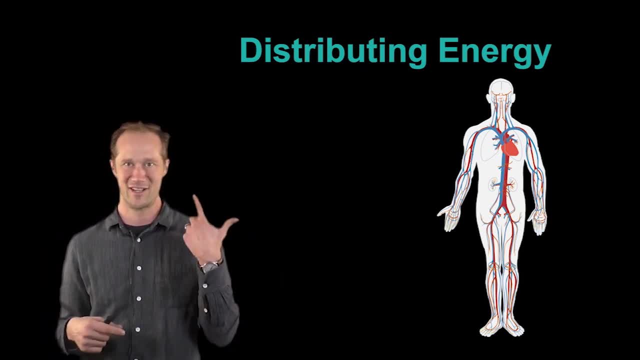 we still have to get it to the rest of our bodies, to our fingertip, our toe tip, our head to use, And that's done by a branching system inside our bodies. It looks a lot like the branching system in trees outside or in their roots in the ground. 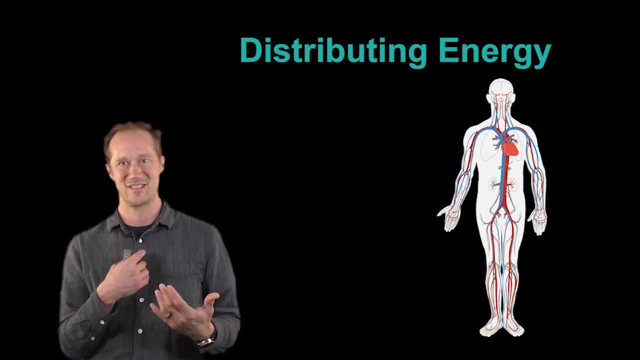 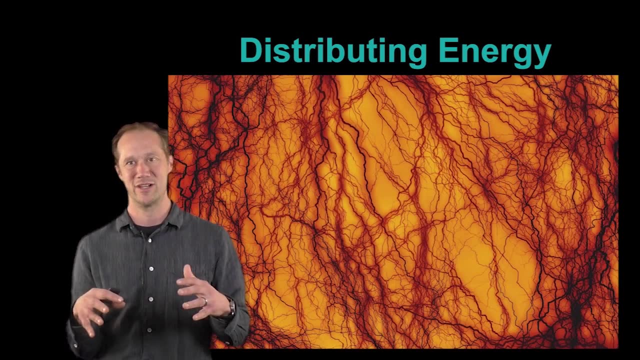 And that's the cardiovascular system, where we use a heart to pump blood out to our limbs and to our head, And then, at the finer scale, we have capillaries or capillary beds, which is where the transfer of oxygen or other nutrients can take place. 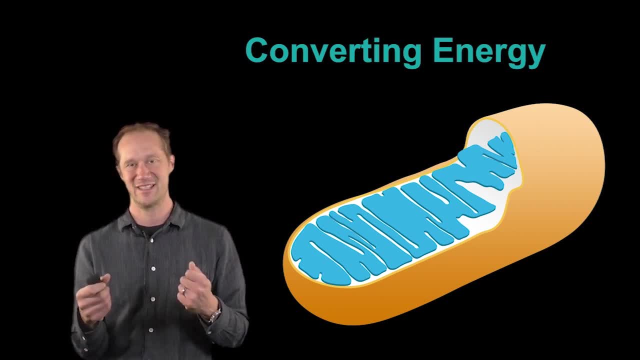 Once we distribute energy and get it to each cell that needs it to keep producing energy and living. the main way we make energy, at least in animals, is through mitochondria, And each mitochondria is like a little engine that takes oxygen and makes energy. 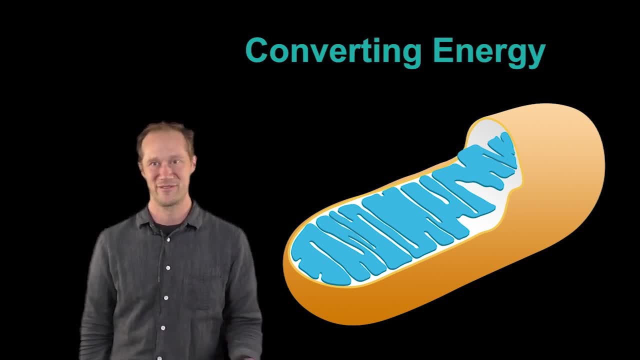 And it's actually a really old bacteria that we've brought into- not we humans, but a long time ago cells brought in to make energy for them, So it's a really ancient way of making energy. And that begs the question of if it's really ancient, is it really good at it? 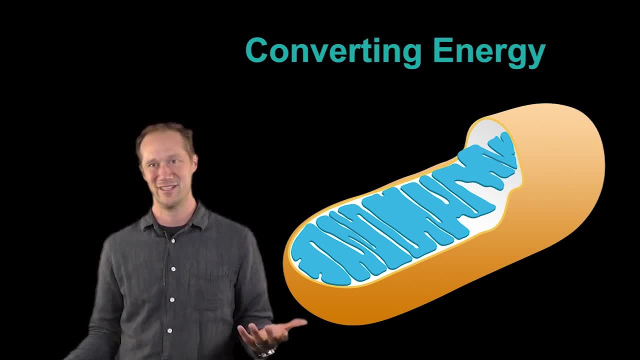 Is it very efficient? And I would think it would be, because if it's used that broadly, you would think it must be pretty good or you would reinvent the wheel somehow. But what's interesting is if you compare to something like solar panels. 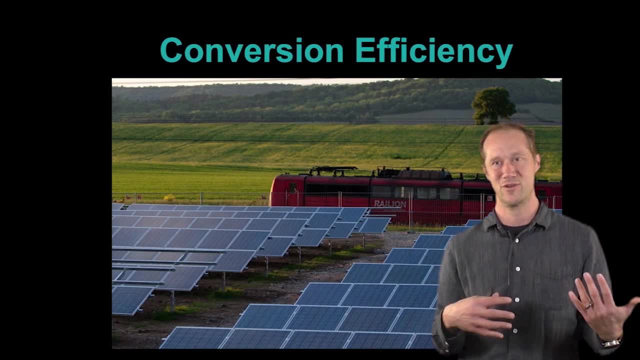 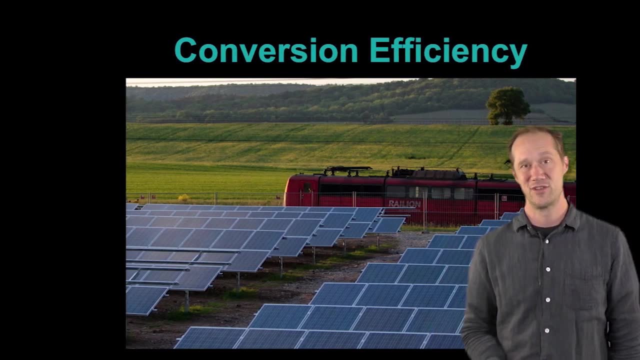 and compare the grass and the trees in the background here to the solar panels in the foreground. the grass and the trees use photosynthesis to make energy, which is about 3% effective, But the solar panels can get up to about 30% efficiency, so about 10 times better. 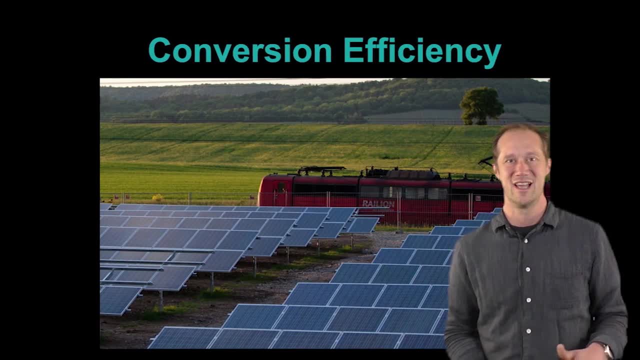 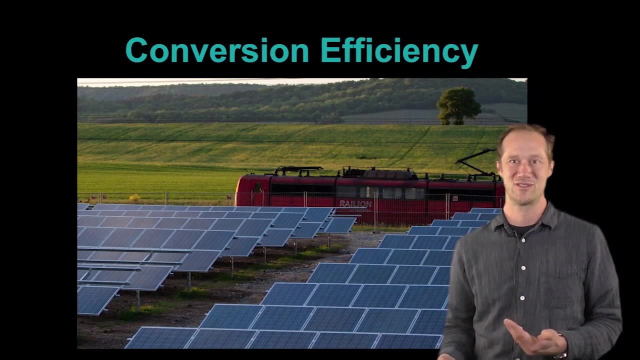 which was kind of shocking to me when I first learned about it. they can do so much better, And maybe this does suggest that biology can still evolve and do better. But the catch here really is that solar panels use a lot of elements that aren't easily accessible to biological organisms. 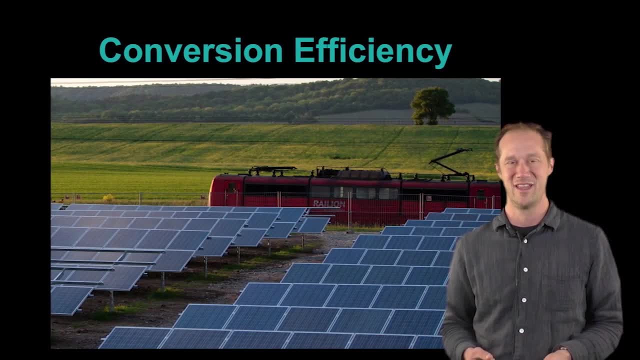 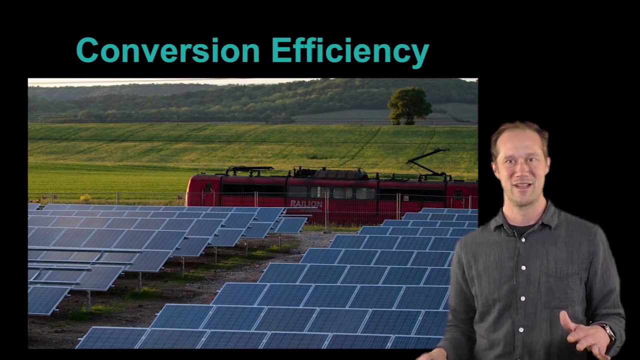 And they take money to either mine or to construct in the right way. So when we think about sort of being efficient or evolving, it's always within constraints. So I'd argue biology's probably done really well within the constraints it has, but we're able to get at things biology has not been able to get to. 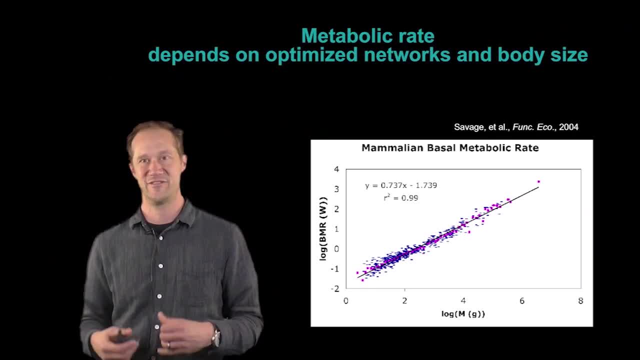 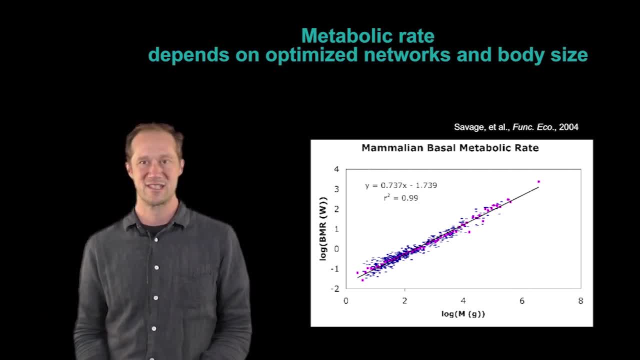 there's a million ways you could build such a network. We want those networks to span space, to be able to get blood or water everywhere it needs to go, And we want them to do so in an efficient way so we don't spend a huge amount of energy just pumping blood around. 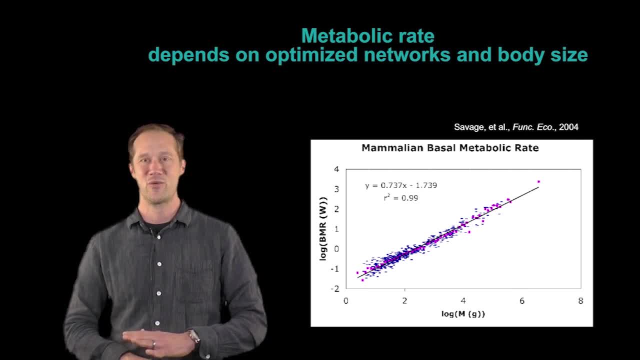 and losing energy to pushing fluid around. And if you think about all the ways in which networks could be built, you can drive theory and look at data to see what's the most optimal, And it turns out that biology has done a really good job of optimizing networks to be efficient. 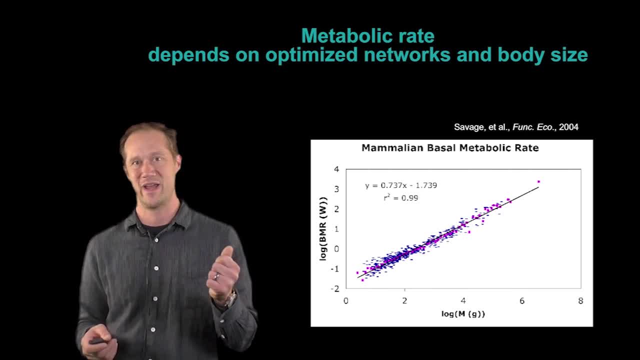 And one consequence of that. actually, if you look at metabolic rates on the y-axis here versus mass on the x-axis, you see a very clean systematic pattern where the bigger something is, the more energy it uses, which isn't surprising. 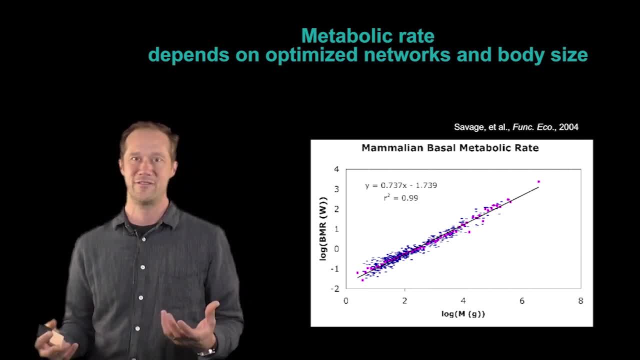 But the surprising piece here is that it's nonlinear. So if you think about an elephant, that's 10,000 times bigger than a mouse. it only uses about a thousand times more energy, which means per cell. a cell from an elephant uses about 10 times less energy than a cell from a mouse. 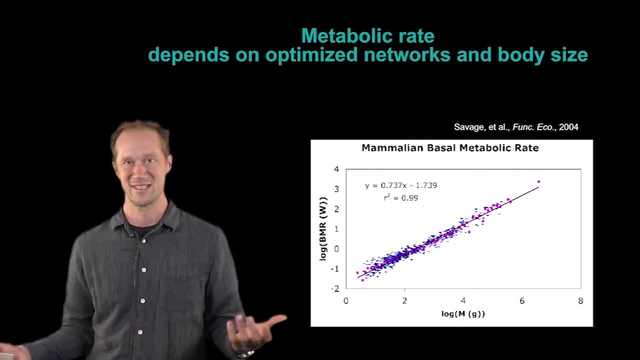 So you're gaining efficiency by getting bigger in this way of looking at it. And just to make sure for people paying close attention to the axes here, they're logarithmic axes, So a curved line becomes a straight line and what would be the exponent in a mathematical equation becomes the slope. 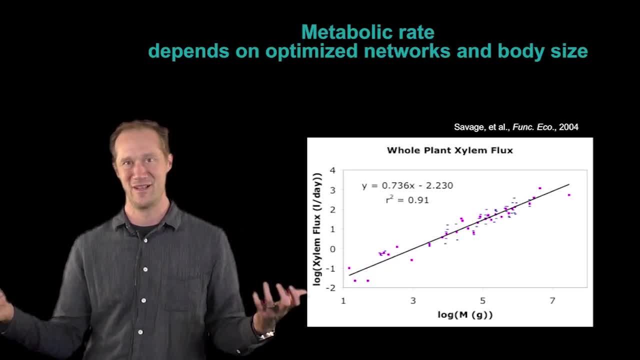 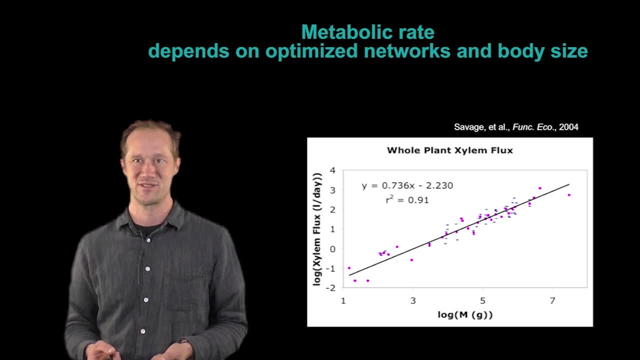 And this pattern is true not just for across these large, huge range of sizes in mammals or animals in general, but also for plants. Silent flux is a similar sort of measure of metabolic rate in plants. We plot that versus body size. again And again you see a very clear straight line across a huge range in size for plants. 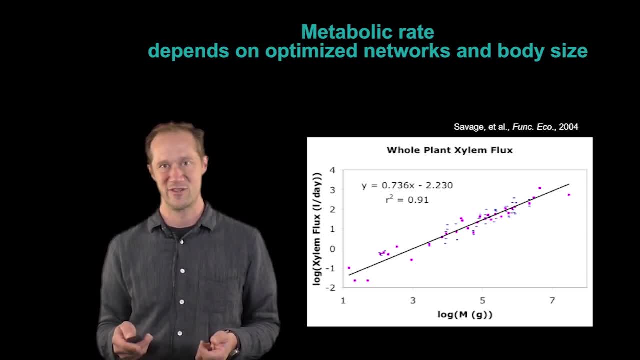 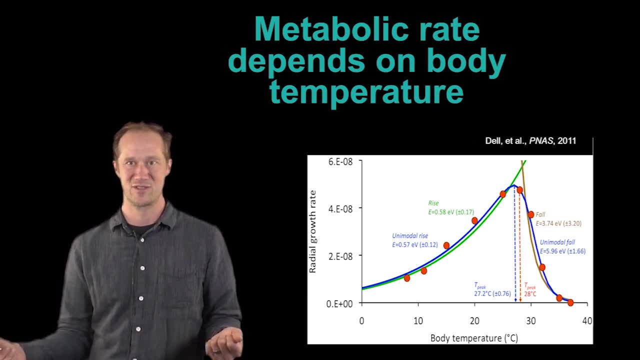 And again an exponent or a slope that's close to 3-4.. So the same sort of pattern shows up again. And another big effect here: besides body size: after body size, the biggest effect of energy use across individuals is temperature. 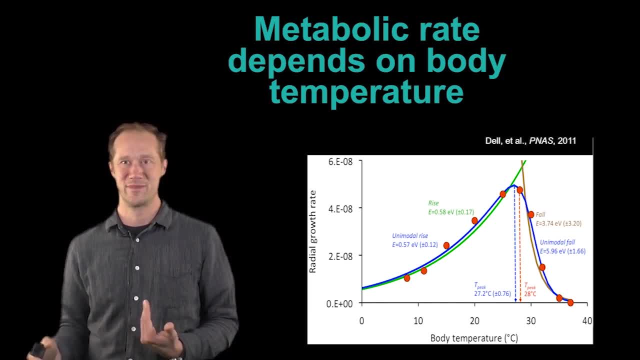 So if you look in this figure, basically the warmer something is if you think about a frog or a turtle or a plant, the warmer it is, the faster it uses energy And that increases at an exponential rate. so faster and faster and faster. 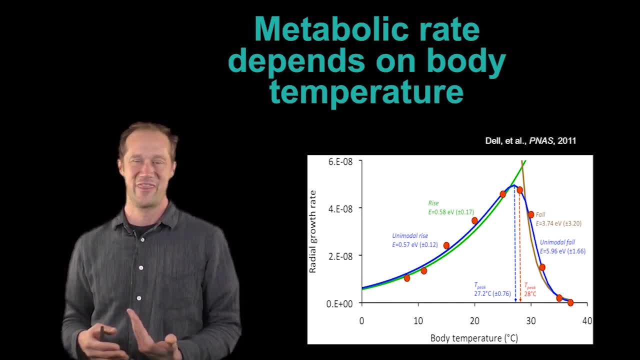 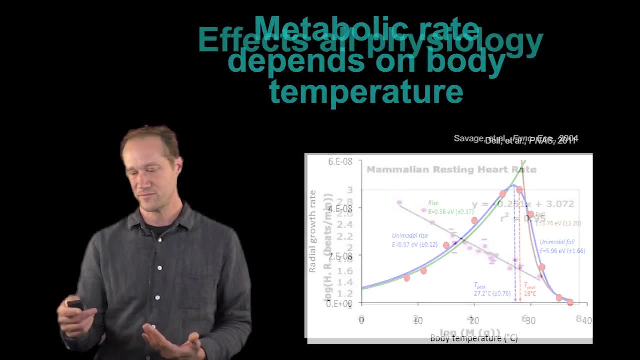 up to the point where you get extreme temperatures and things start to fall apart and things just start to die. But up until that point, or close to it, the warmer you are, the faster you use energy And because, as we started saying at the start of this talk, that we use energy for everything we do, 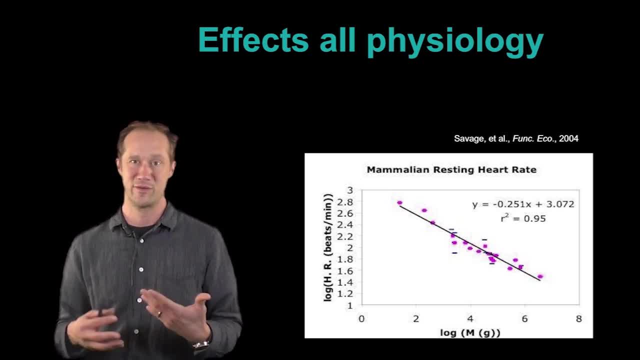 understanding how mass and temperature affect metabolic rate or the power we produce, tells us a lot about all kinds of other things in biology. So, for example, if you look at heart rate across mammals- another way to think about this- in terms of mouse versus elephant-